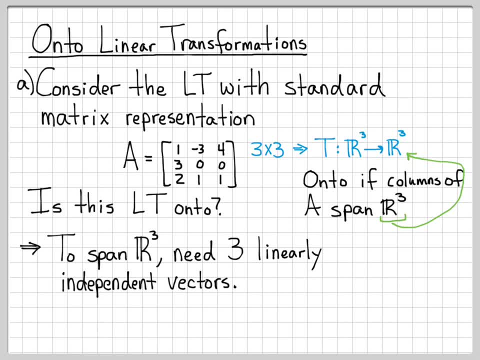 So if these vectors are going to span R3, I really just need to make sure that they're linearly independent, Because I already have three vectors. There's three vectors right here. So, answering the question, do these columns span R3, boils down to: are these three vectors? 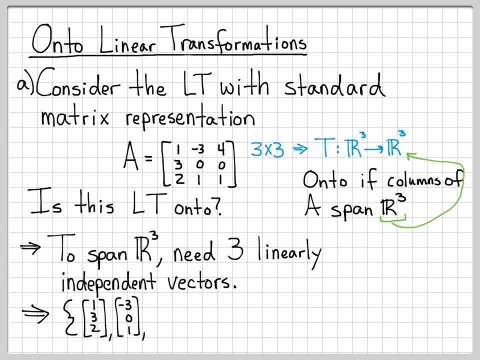 linearly independent. So is this set of vectors- 1, 3, 2,, a negative 3, 0, 1, and 4, 0, 1, are these linearly independent? That's the question we need to answer. 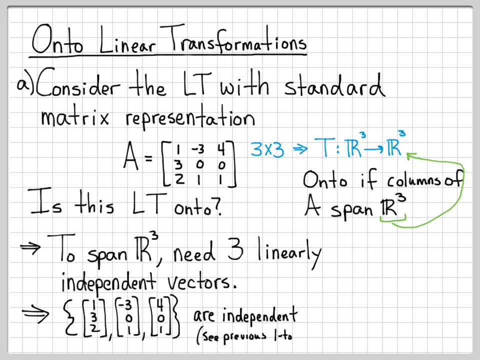 They are independent. In the previous video, the one about one-to-one linear transformations, we actually went through the math And we figured out that when we construct an augmented matrix Corresponding to the homogeneous system of equations for this matrix, we end up getting 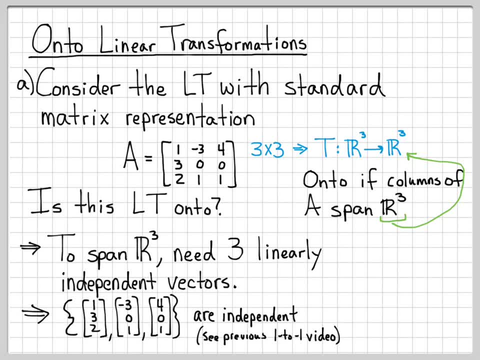 just the trivial solution, And that tells us that these vectors are linearly independent. So, since these vectors are linearly independent- and there are three of them- we know that they span R3.. Since they span R3, that means that we can reach any point in R3 that we would like by 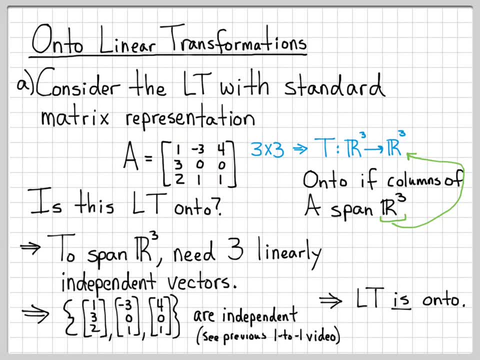 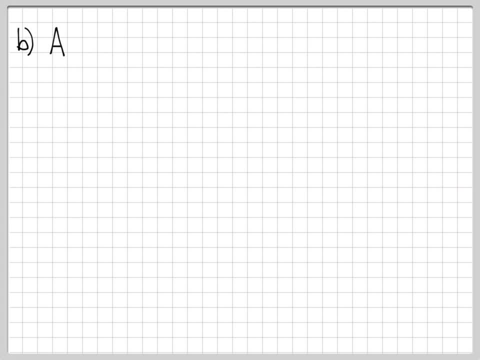 choosing coefficients to weight and sum these vectors appropriately. So this linear transformation is going to be very difficult. So the linear transformation is onto. Let's take a look at another one. So this is going to be the same matrix we saw before. I've just changed this element, just one element, to 3.. 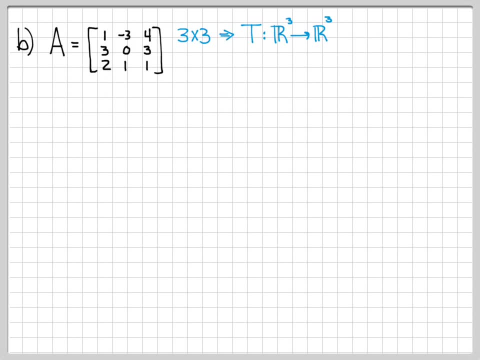 We're going to ask the same question: Is this an onto transformation? Again, this takes elements from R3 to R3. And we want to know: is it onto, Which means? can I reach any point in R3 here that I would like? 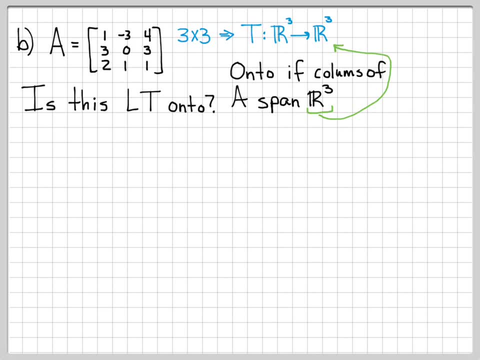 So, equivalently, we're asking: do the columns of A span R3? Yes or no? To figure out if they span R3, I can determine that by figuring out if I have three linearly independent vectors or if I have three linearly dependent vectors. 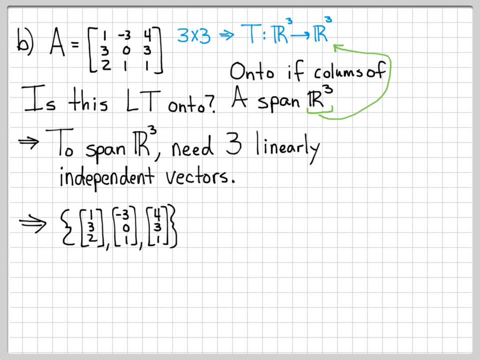 So again, the question is: given this set of vectors, are they linearly independent or linearly dependent? These are not independent. Again, in the previous video we went through the math. We constructed an augmented matrix corresponding to the homogeneous system of equations.